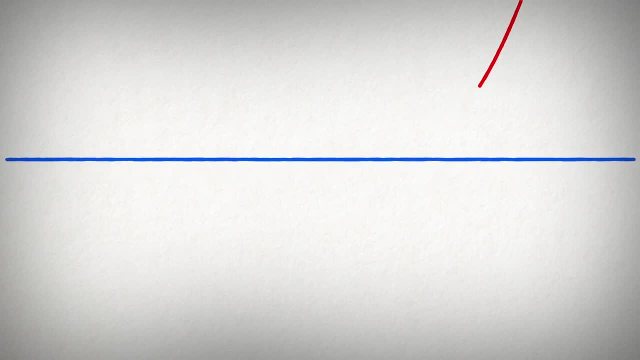 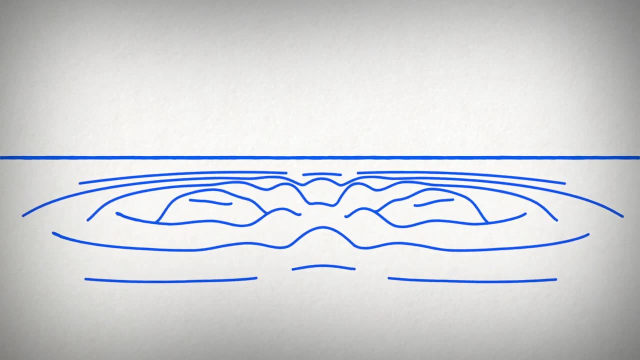 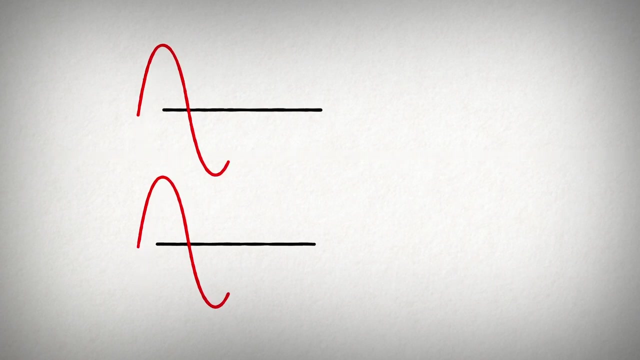 To understand x-ray diffraction we first have to look into wave properties called interference. Very similar to throwing two rocks into the water, the circular ripples that result from the two stones seem to pass through one another as they propagate out from where the stones entered. This is known as interference. 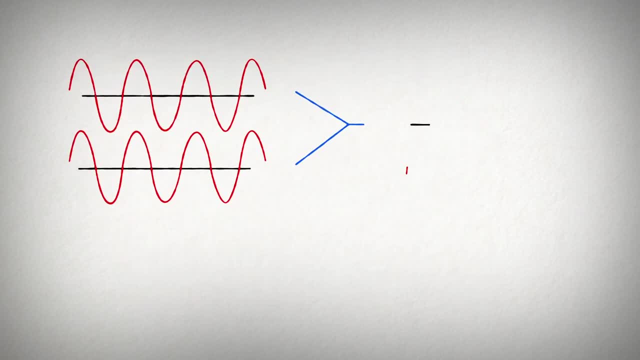 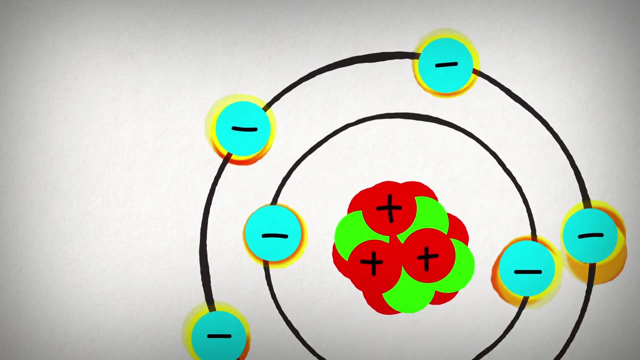 If the waves are in alignment, the signal is amplified. This is called constructive interference. If the waves are out of alignment, the signal is destroyed. This is called destructive interference. When an X-ray encounters an atom, its energy is absorbed by the atom's electrons. 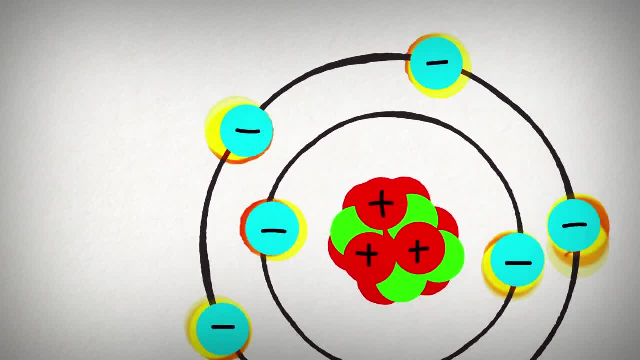 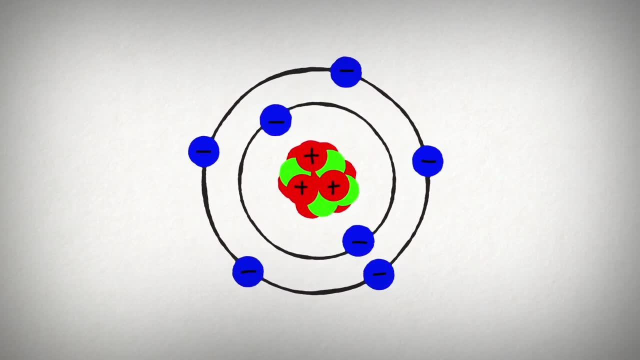 Electrons occupy special energy states around an atom. Since the absorbed energy is not large enough to release the electron, the energy must be re-emitted in the form of a new X-ray with the same energy as the original. This process is called elastic scattering. 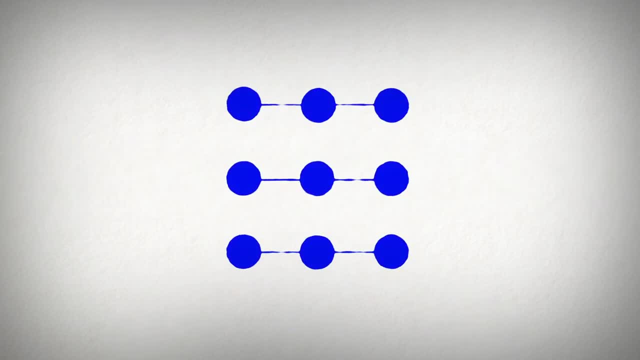 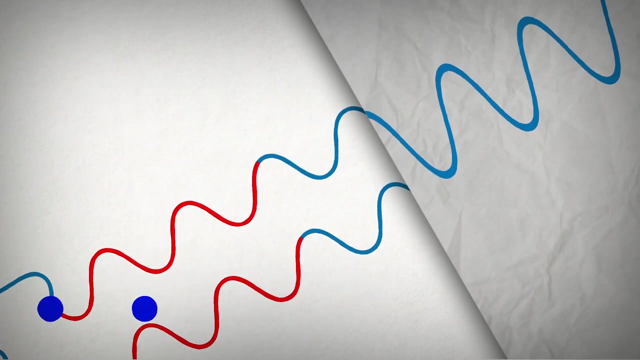 In a crystal, the repeating arrangement of atoms, ions or molecules forms a lattice with well-defined repeating distances. When planes in these lattices are exposed to an X-ray beam, X-rays are scattered by this regular arrangement. Strong amplification of the emitted signal occurs at very specific angles, where the scattered 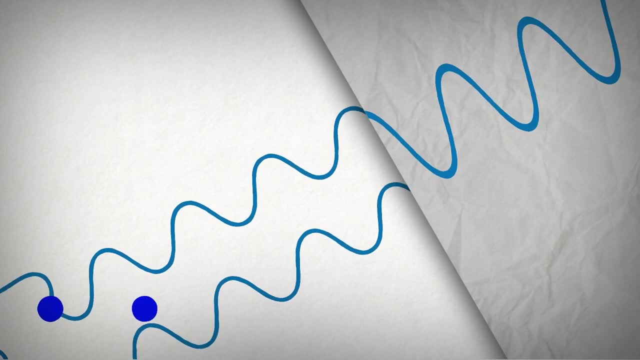 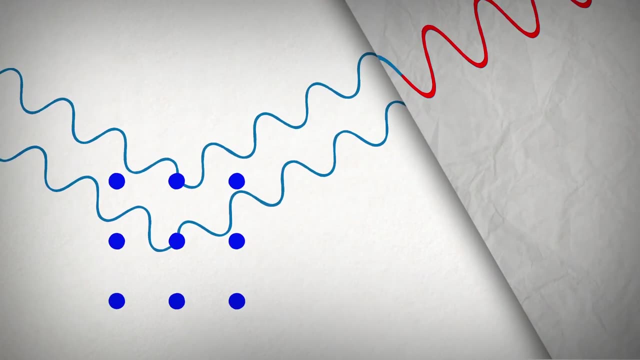 waves constructively interfere. This effect is called diffraction Subtitles by the Amaraorg community. The angle between the incident and scattered beams is called 2 theta. For constructive interference to occur, the scattered waves must be in alignment, meaning the second wave must travel a whole number of wavelengths. 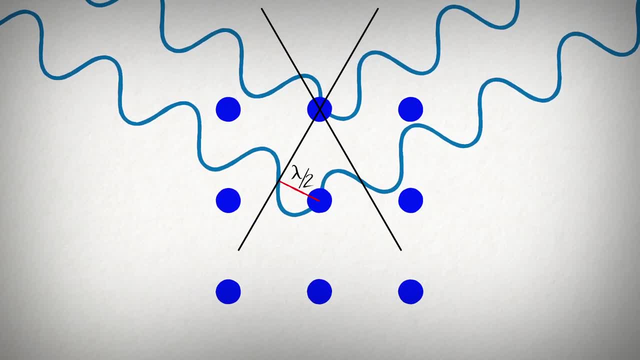 In this case, one half of a wavelength is traveled on the incident side and one half of a wavelength is traveled on the scattered side, resulting in one additional wavelength. In the case of the next X-ray, one wavelength is traveled on both the incident and the scattered. 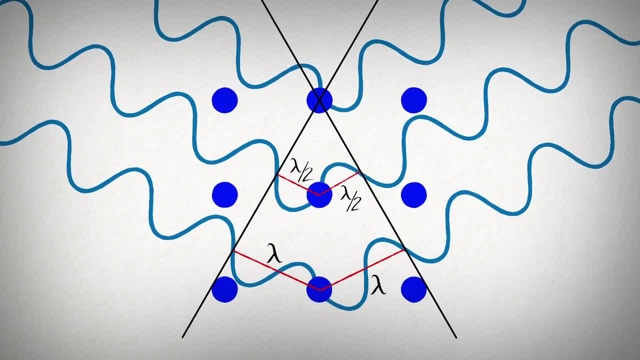 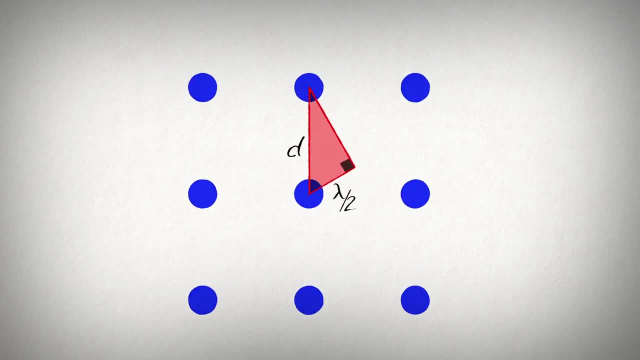 sides, resulting in two wavelengths. This reinforcement occurs throughout the crystal. The exact angle at which diffraction occurs can be determined from the red triangle. The angle at the top is theta half the angle between the incident and scattered beams. The long side is the distance between the atomic planes and the short side is one half. 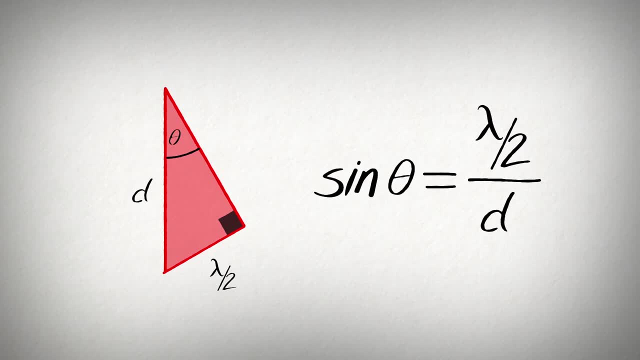 of a wavelength. The relationship between the diffraction angle and the spacing between the atoms can be determined by applying the sine function. Rearranging this equation yields an equation commonly known as Bragg's law. The equation is defined by the function of the distance between the incident and scattered.